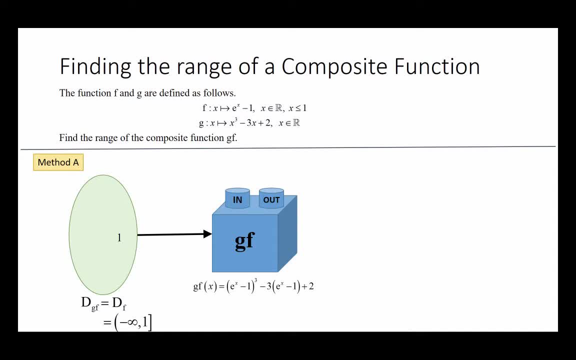 1.. So there are a few examples of values that can be found in this domain, such as 1,, 0,, negative 1,, and so on. Then let us look at an example of fitting one value from this domain into our. 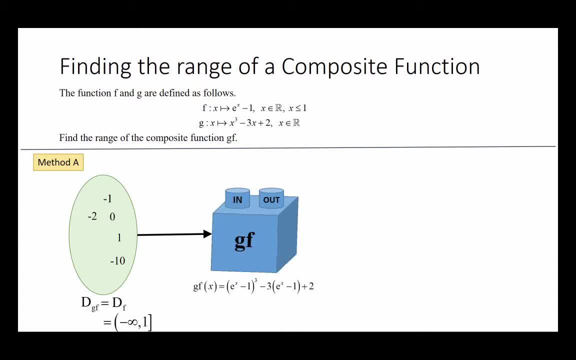 machine. Let's say we take 0, put it into our machine of gf and put it into our machine of gf. Then let us look at an example of fitting one value from this domain into our machine of gf. We can see that gf will work on this value and come up with an. 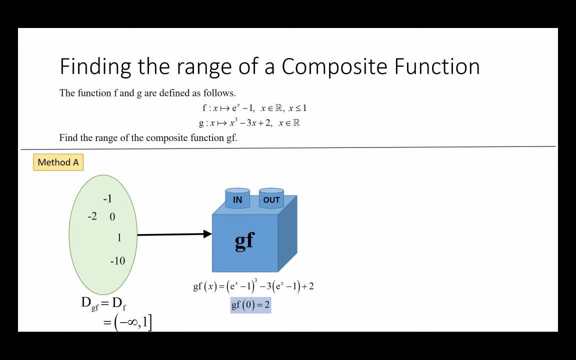 output, in this case, which is 2.. This output will form a set of values that is being known as the range of gf. Similarly, if we input the value of negative 1 into our machine, it will work on this value and come up with an output, in this case, 3.64.. Again, this value. 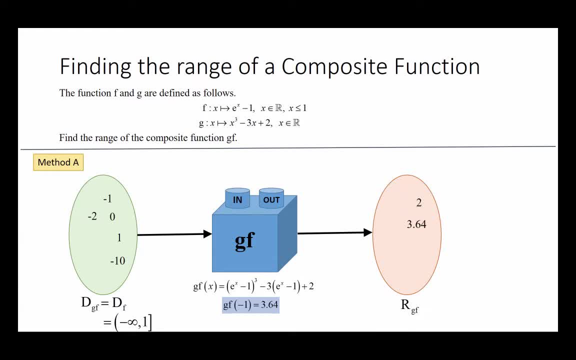 will form part of the set of values known as the range of gf. This will follow, for the same as the other values that we have given as examples from the domain of GF. So how does this works mathematically? Step 1, we find the rule and domain of. 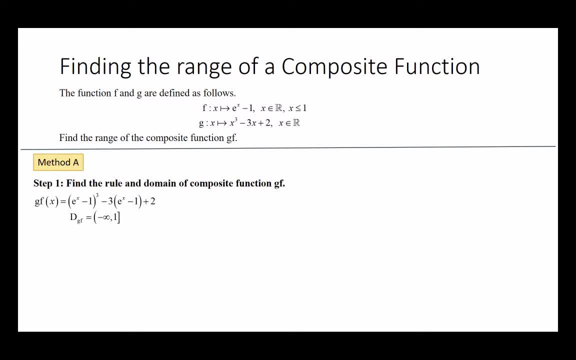 the composite function GF, first, as shown on the screen. Next, we draw the graph of GF within the domain that we have found. You can use your GC to help you to sketch this graph. From the graph we can easily see what is the range of this. 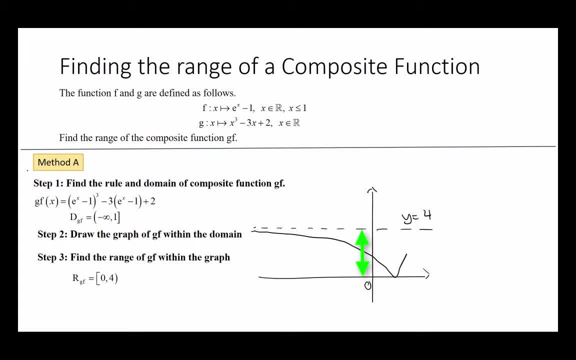 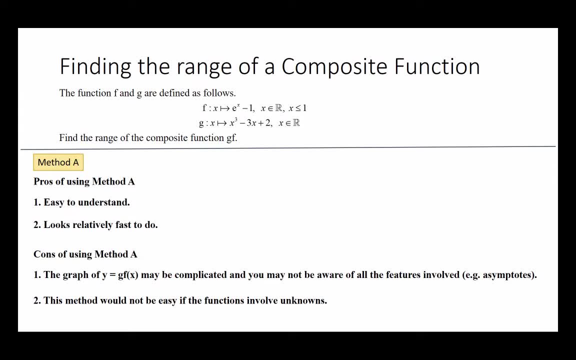 composite function, in this case, which is going from 0 to 4.. There are a few pros and cons of using method A, as shown on the screen. You can spend some time to read through these pros and cons. Next we will move on to method B. In this method, we will still start off with the 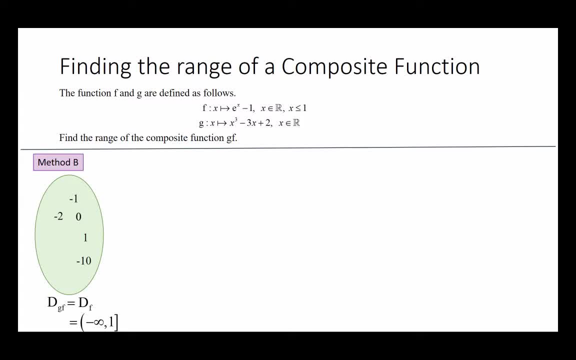 set of values, which is the domain of GF. that is the same as the domain of F, but it is not the same as the domain of GF. So we will start off with the set of values, which is the domain of GF. that is the same as the domain of F, but it is. 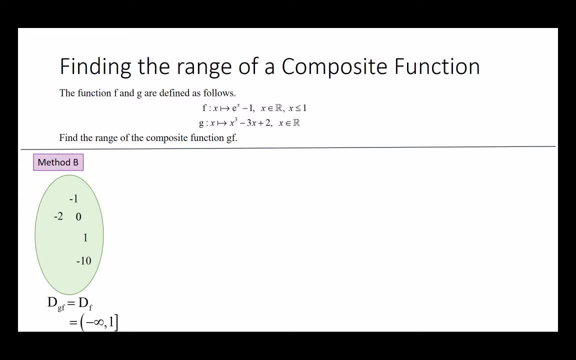 set of values, which is the domain of GF, that is the domain of F, but it is instead of looking at the composite function as one single machine and now we will see as the machine that consists of two separate components. The first component will be the first function that will acts on the values, which is 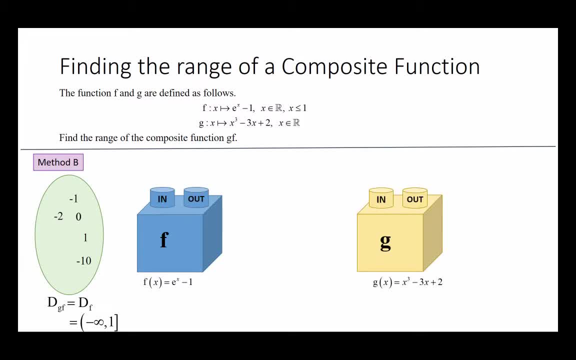 the function F, and the second component is the second function that will act and that will be the function G. So in this case, first we will take a value from the domain of GF, from, let's say, 0, and this will goes into the. 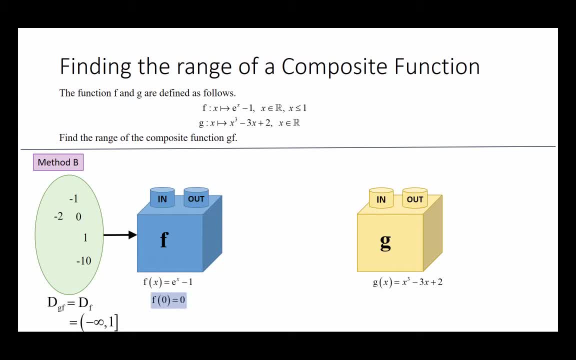 component of the machine, function F first, which will come up with an output, in this case which is 0, this output value is definable, sort of out, as equal c0,. circular output will go into the set of values known as the range of f. 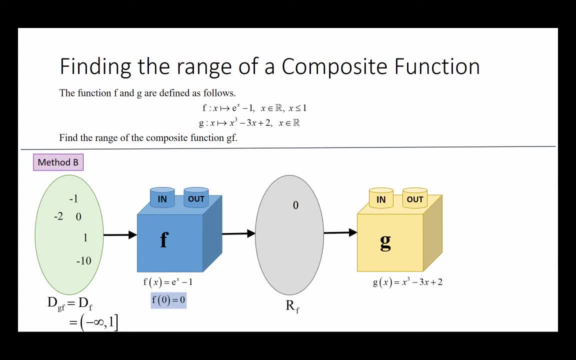 Then this value from the range of f is being fed into the second component of the machine, which is function g. This function g will add on this value and come up with an output which is 2 in this case. This output will form the set of values which is known as the range of gf. 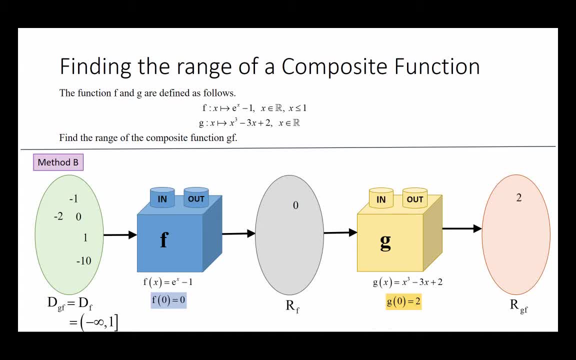 Next, let us look at an example of using the value negative 1 from the domain of gf. If we feed negative 1 into the function f, it will work on this value, come up with an output and this output will form part of the range of f. 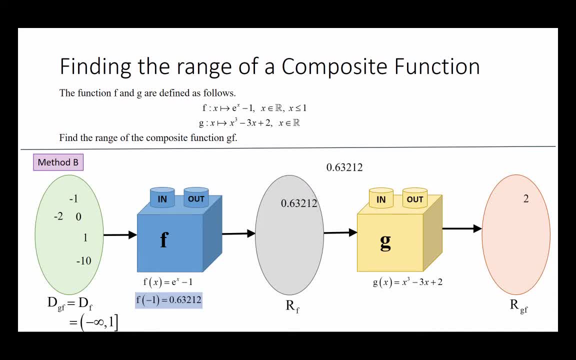 Then the function g will take in this value from the range of f, works on it and have an output. This output will form the set of values known as the range of gf. This will work on the domain of gf The same way for the rest of the values given as an example in the domain of gf. 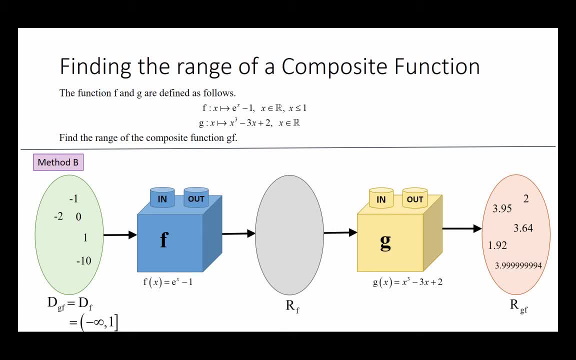 As you can see, these values are exactly the same as those that we have found in method a. How do we do this mathematically? First, we find the range of the function f. This corresponds to the first components of the machine, as we have seen earlier. 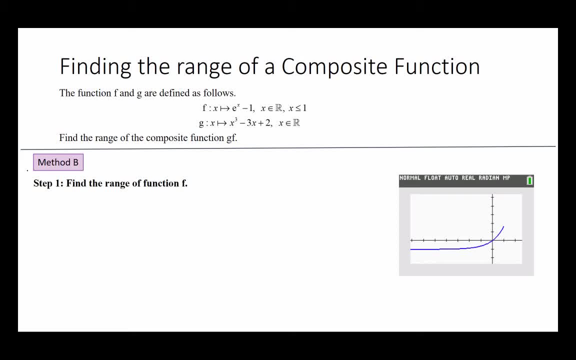 To find the range of function f, we will draw out the graph of y equals to fx. We can use our gc to help us And from the graph we can easily see that the range of f is from negative 1 to e-1.. 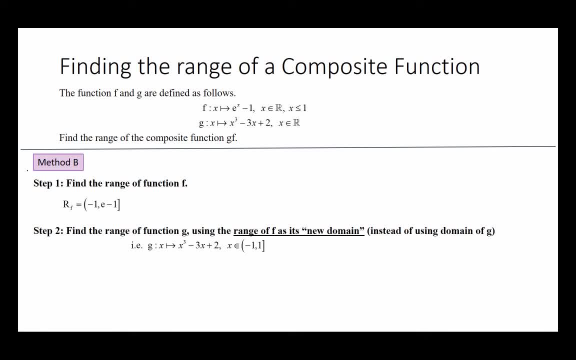 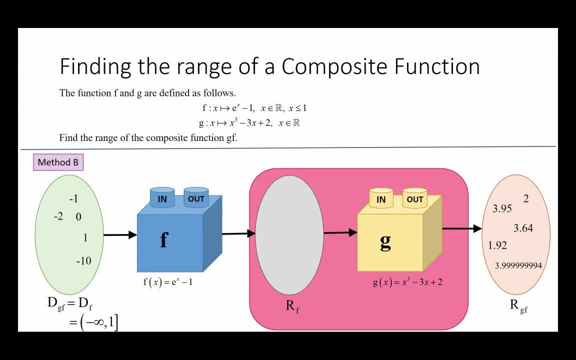 Next we will find the range of the function g, but instead of using its own domain, we will use the range of f as its new domain. This corresponds to the second component in our machine. As you can see in this diagram, g doesn't act on its own domain anymore, but instead. 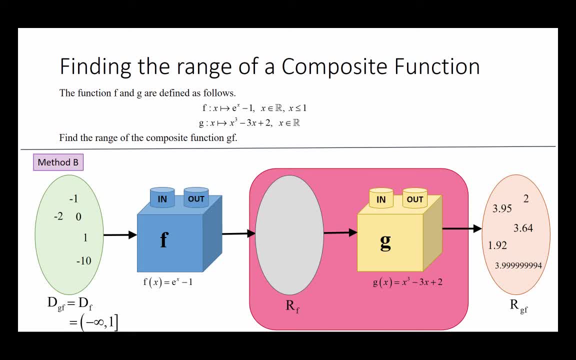 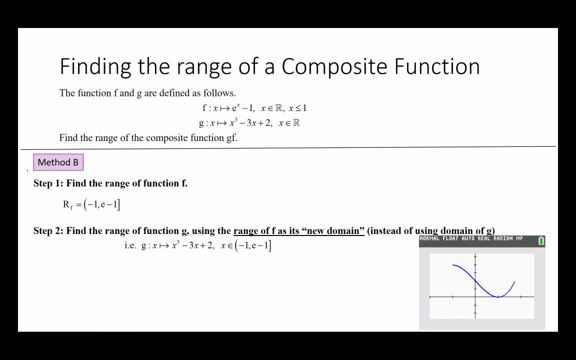 g acts on values. that is taken from the range of function f. As we can see on the graph that has been drawn using the gc, we have the graph of y equals to gx. that does not go for the whole domain of g. Instead, it only goes from negative 1 to e-1, which is our range of f.